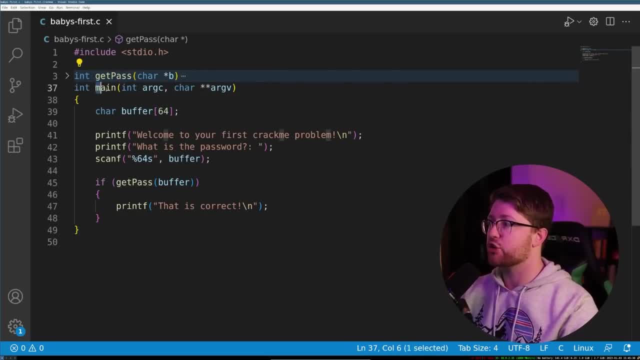 code. I have a bunch of different symbols in the binary that are human-readable. I have the type of the variable, I have the name of the function, I have the name of the variable, etc. All of these symbols, these human-readable strings, these labels tell me what the code is going to do. 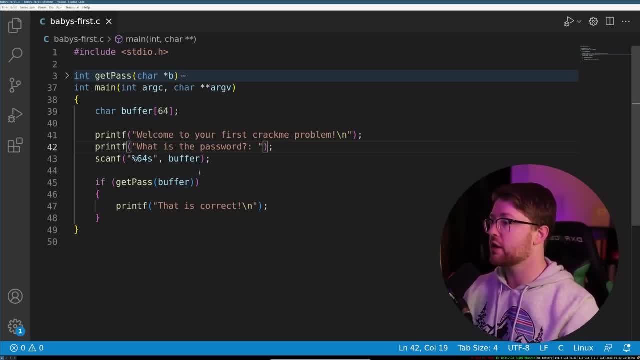 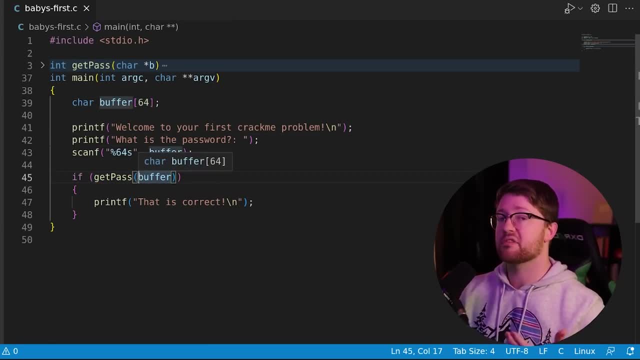 I can infer a lot of information from the source code by reading the code. For example, I have a buffer that gets passed to scanf and then I call getPass on that buffer Because I have the source code. I now know generally that I will read in data from the. 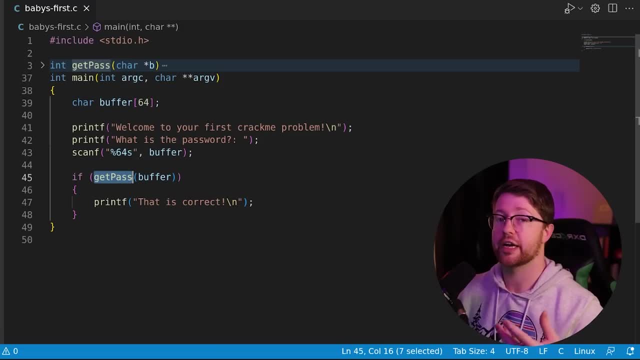 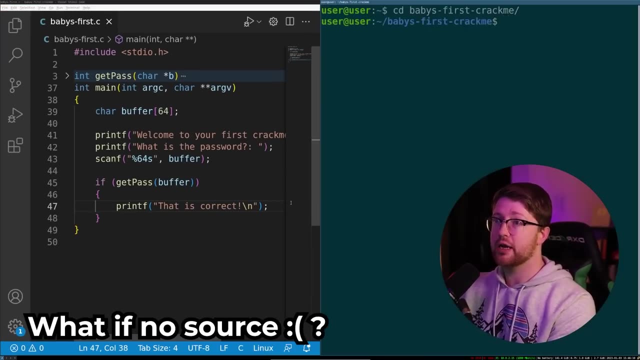 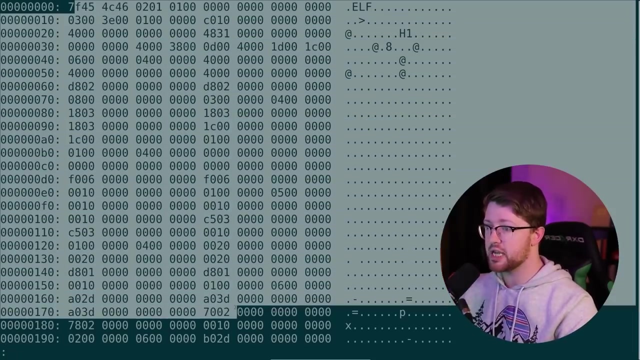 user and I will check that buffer against a known password. If I get it right, I get to go to the. that is correct block. The problem is that if I have just the binary, I don't have that source code. Instead, what I have is this really horrific binary blob of data. 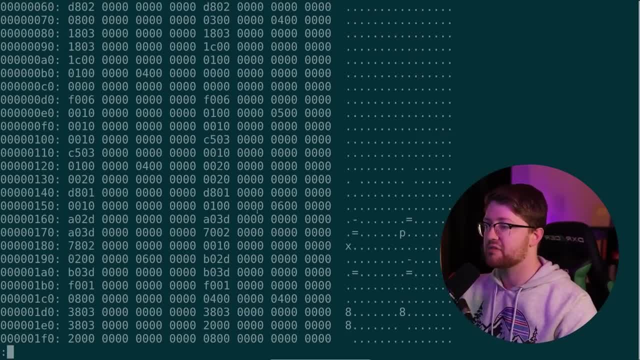 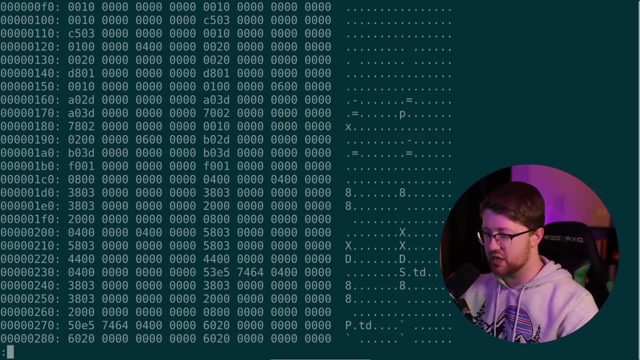 that, looking at this, I can't infer any information about this. Reverse engineering is going from this without the source code and inferring the features from what the code does. Why do we do that in the first place? The number one thing, I think, is for cybersecurity. 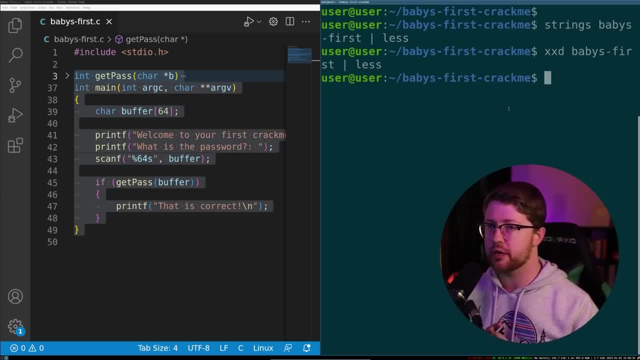 professionals. the art of malware. reverse engineering is extremely important for a few reasons, The big one being if you're able to take the malware that you find in your system and triage it by hand, instead of depending on a sandbox analyzer, you can yourself. 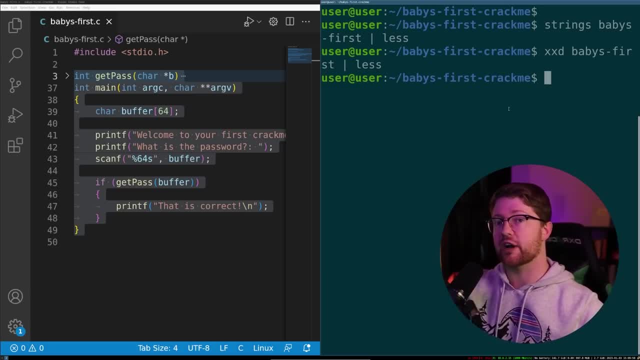 figure out what the attacker was trying to do and then from that infer how to defend against it. Number two: I think reverse engineering is just fun. I think the art of taking things that you don't know what they do, looking inside of them and figuring out. 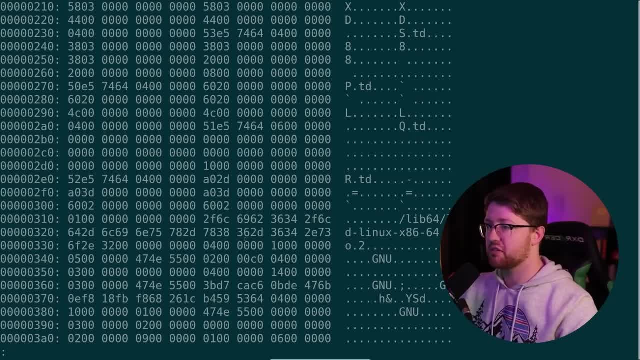 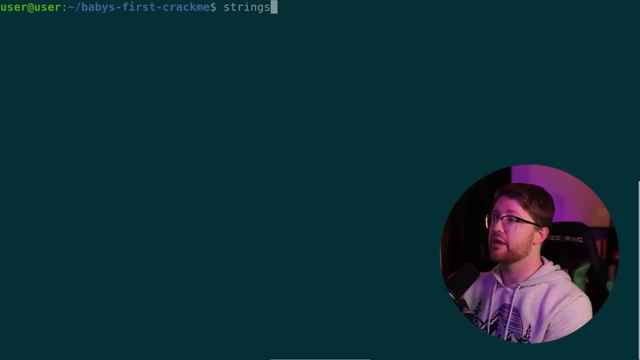 what they're supposed to do is really fun. There's a couple different techniques that we can do to reverse engineer this binary. The first one that everyone can do right now on your computer is we can do the operation strings on our binaries. We're going to do that. 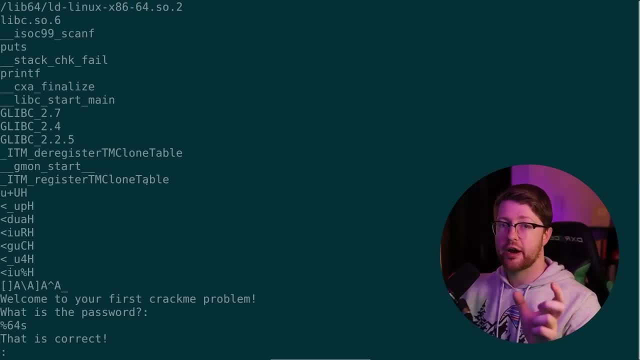 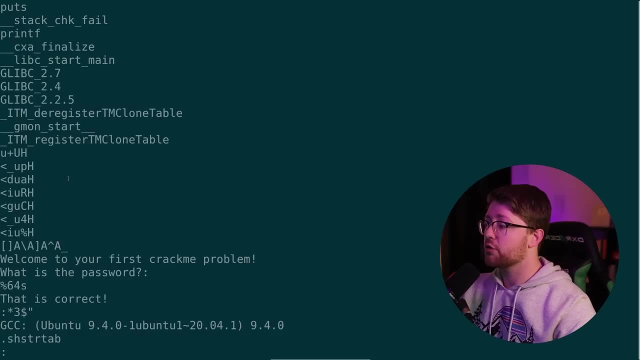 All the strings Benutil does is it looks for a five character or greater string of ASCII characters and prints them to the screen if they're found in the binary. These are all the strings in the binary. You can see we have the name of the functions that we import like scan. 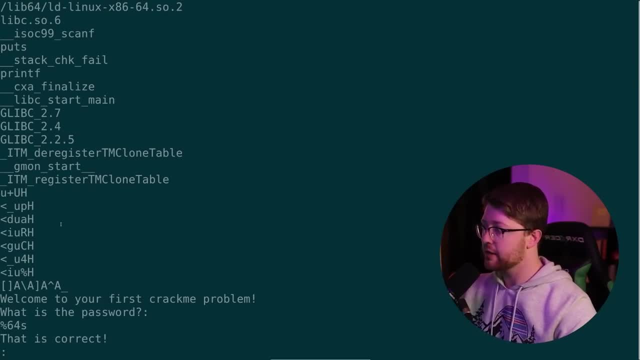 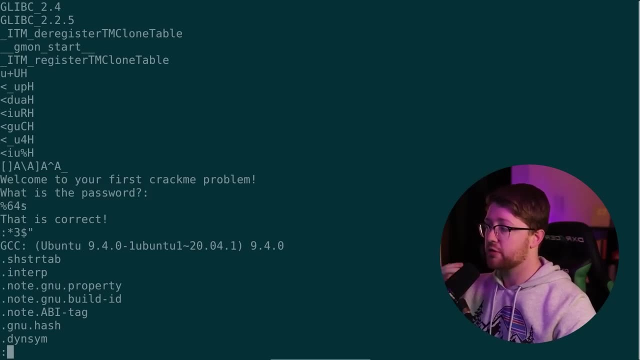 f puts and print f. Those will always get preserved for the reasons of linking. Then we have the strings we actually wrote into our program. We have welcome to your first crack me problem. What is the password, The format string for the scan f, and then that is correct. 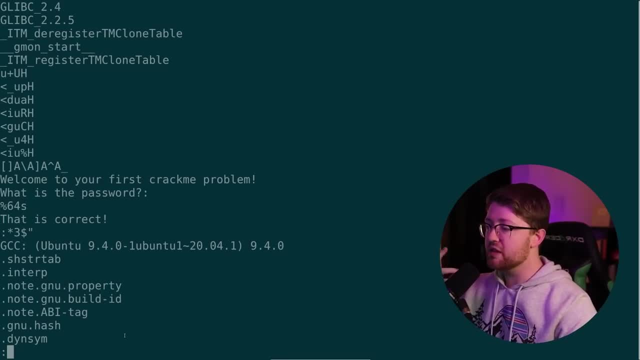 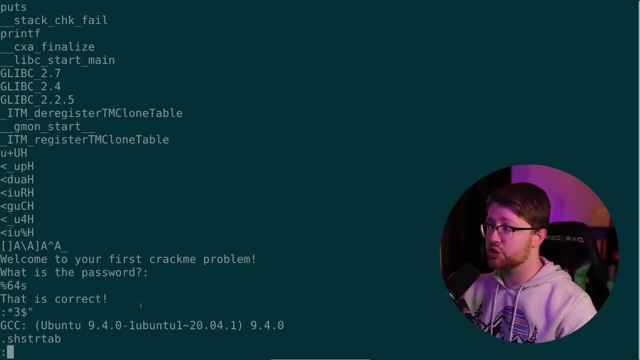 The problem with this is that the password itself is not revealed in the binary. We have to go through the art of getting a little deeper, reading the machine code and figuring out what the machine code does to get the password from the user Going one level deeper instead of strings. 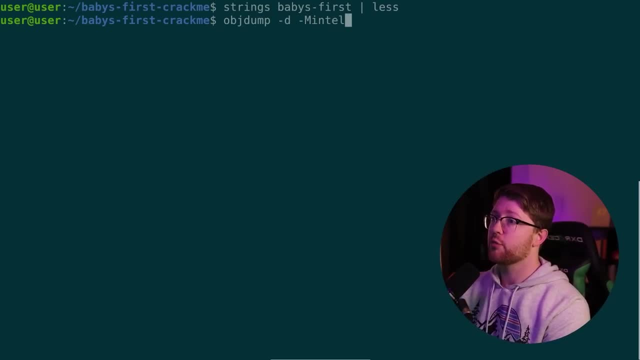 we can kind of put this in the binary. We can kind of put this in the binary. We can kind of put this into what is called a disassembler. The one disassembler everyone has access to right now is going to be object dump. So we're going to write object dump, disassemble the main sections use. 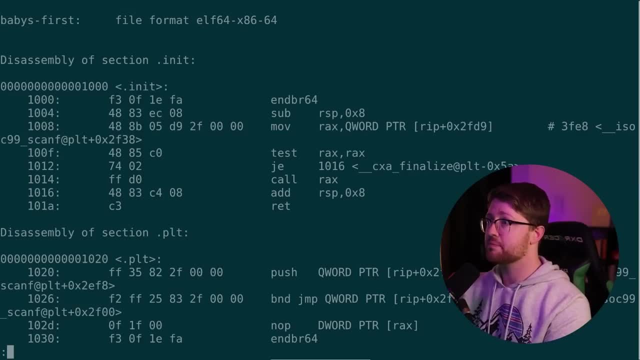 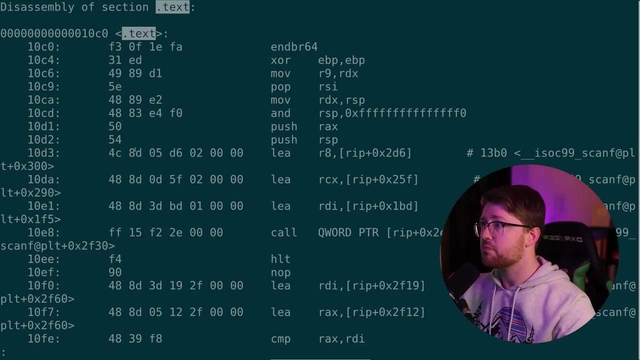 Intel syntax on our program and pipe that into less. Now what we have here is the disassembler is taking the ones and zeros, the literal hex data, and converting that into a human readable version of the assembly instruction. So if we navigate down to the text section, the text section contains the: 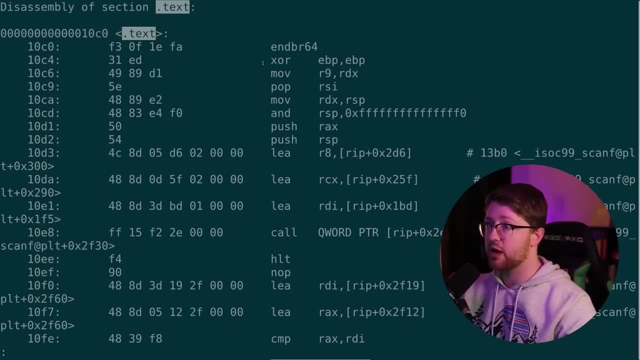 code for our binary right, The executable bits that will get ran by the processor, And here we have the binary data and then the actual human readable assembly instruction. The problem with this now is this is not very human readable. We can probably kind of infer what's happening here. 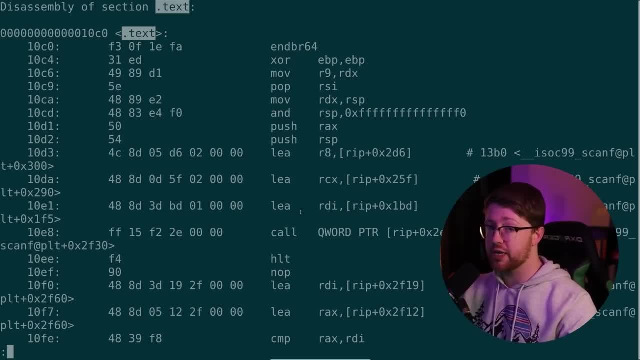 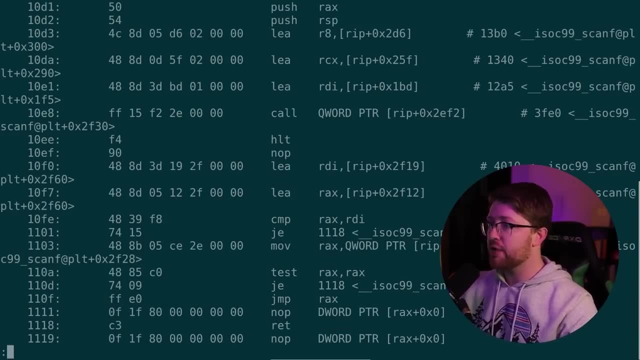 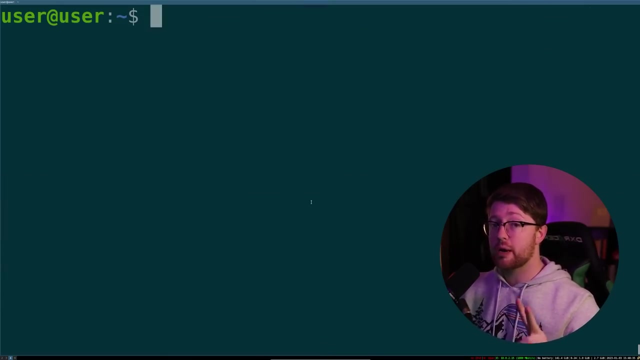 but there's not a good visualization of the control flow graph, meaning the if statements that will either execute or not execute as a binary runs. So we're going to go one level deeper and put the binary into a more complex disassembler And my favorite disassembler. there are two primary ones: There's IDA and Ghidra. I would 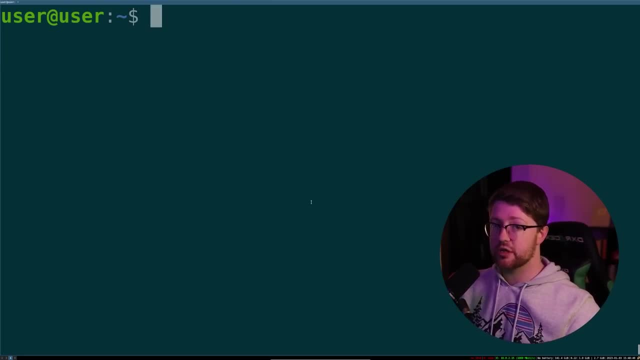 argue, for the reasons of learning assembly and learning reverse engineering, that we should use IDA. So we're going to go ahead and we're going to install that. I've already installed the downloader. I'll put the link for that in the description below. From my downloads you can go. 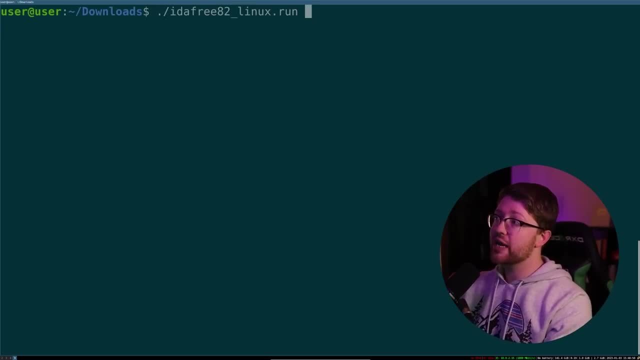 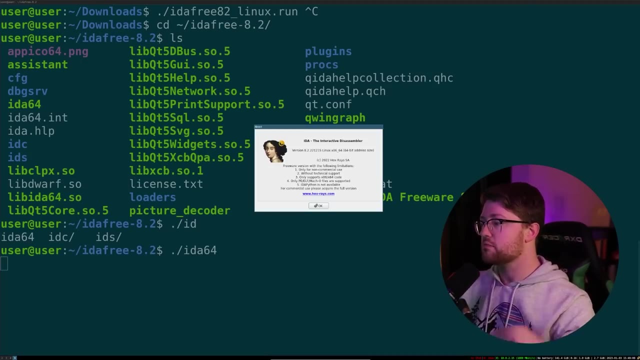 ahead and run the IDA installer And once you've ran the installer, you will get a folder in your home directory called IDA free and we're going to run IDA 64.. We're going to go to baby's first crack. 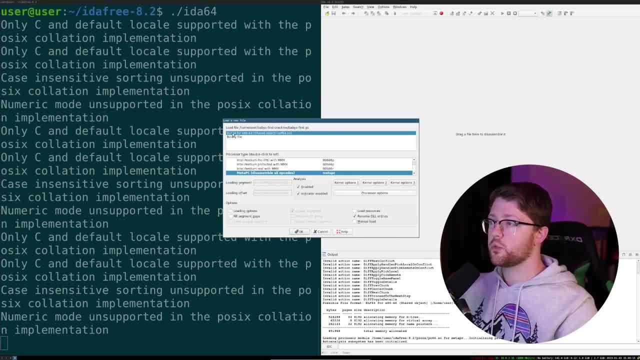 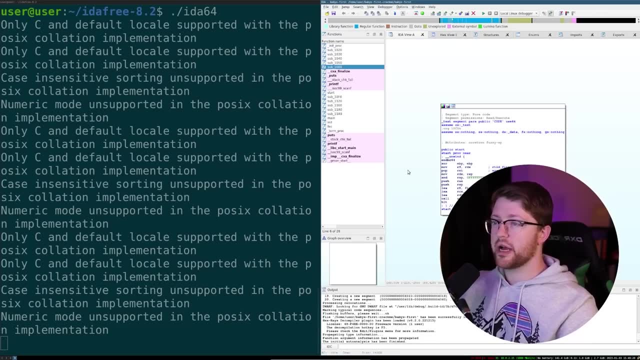 and we're going to import our binary file. It's going to make sure that we are okay with us treating this binary file as an elf 64, and we're going to go ahead and hit okay. What IDA will then do is: IDA will go through and it will disassemble the entire binary. 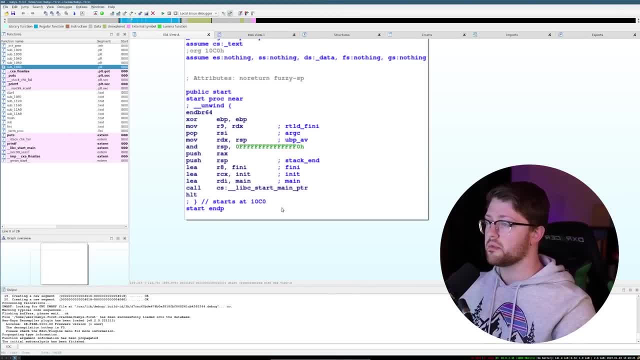 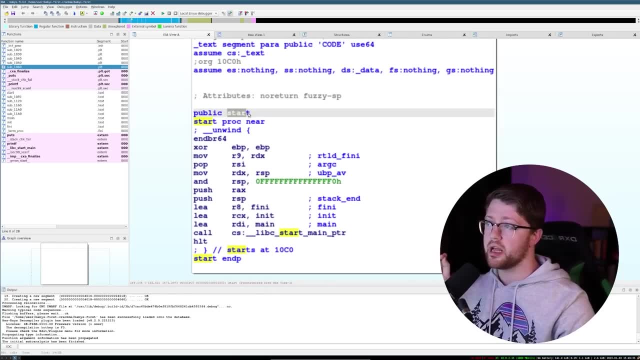 and give us the ability to read the assembly. here I'm going to zoom in on this. And now we are looking at IDA's disassembly of the program from what it inferred as the start point. So the start point is: what is the first instruction that is going to run when the 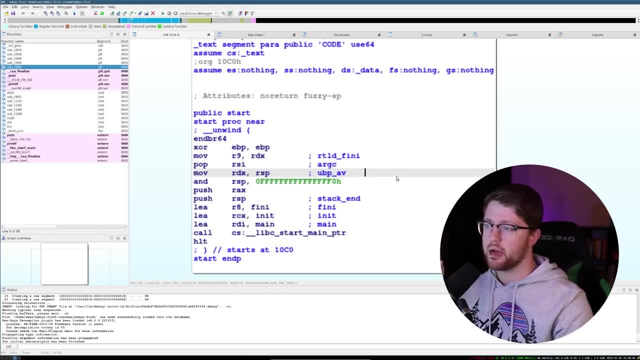 program starts And that's the first instruction that is going to run when the program starts, So starts. there's a lot of stuff here that we can talk about. this is more about the runtime of the libc library initializing. we're going to skip all of this. we're going to jump right into this label. 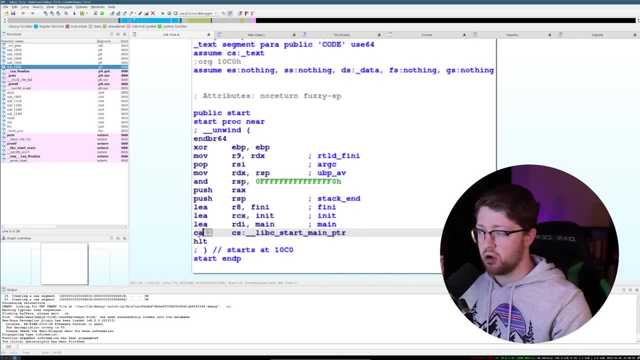 here. so before libc start main gets called- that's what the call instruction does- it loads the effective address of our main function into rdi. so one thing we have to kind of talk about here, very basic reverse engineering concept, is the. is this concept called binary, abis or abstracted? 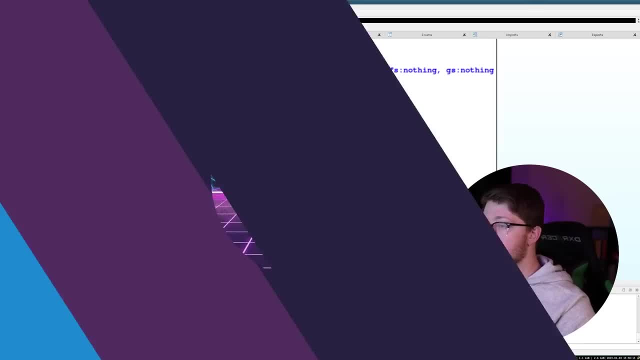 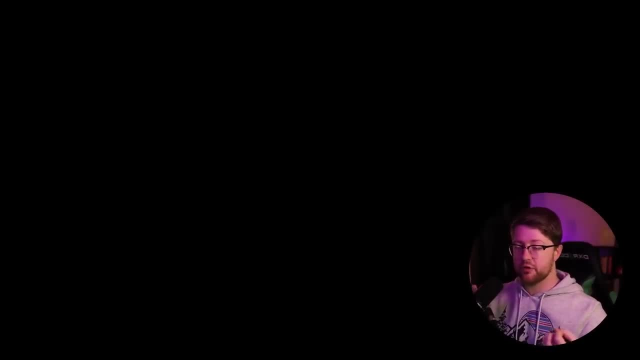 binary interfaces. what these are are the agreement that the computer has made with the processor about the registers that will contain different values and a function is called. so, for example, if i call function foo and numbers one and two are the arguments to foo, before we call foo. 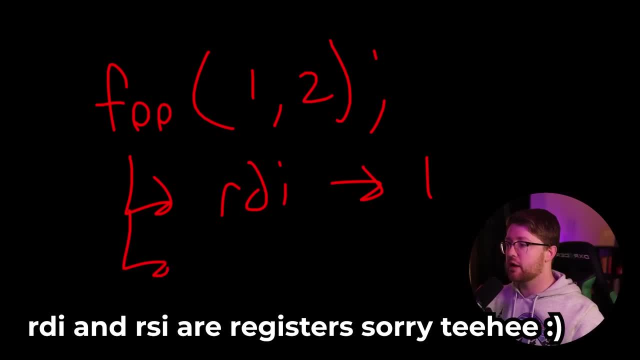 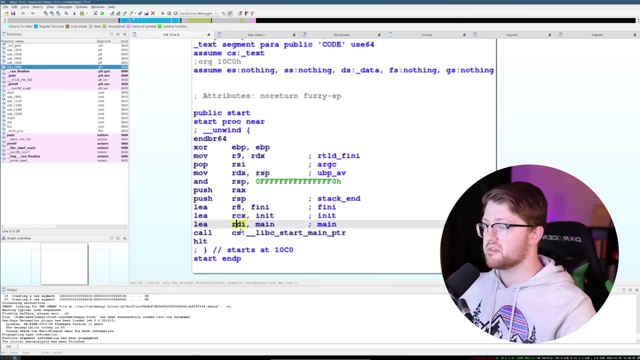 rdi will contain one and then rsi will contain two. this is just the agreement that the compiler has made with the processor, right? this is the way that it expects the data to behave. so if we go back and we look at that, when we call libc start main, we have rdi goes main. 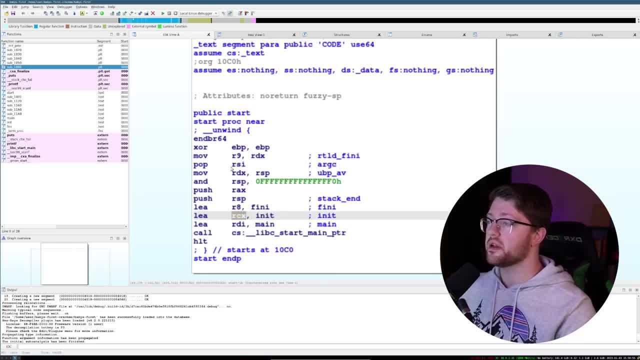 and then- i'm sorry, i guess in this case it's rcx, actually, no, it is rsi. rsi takes arcv, that's the second argument, and then rcx gets the next argument which is in it. so we're going to go ahead and we're going to double click on main and this is our function. that we wrote, you know, before we were. 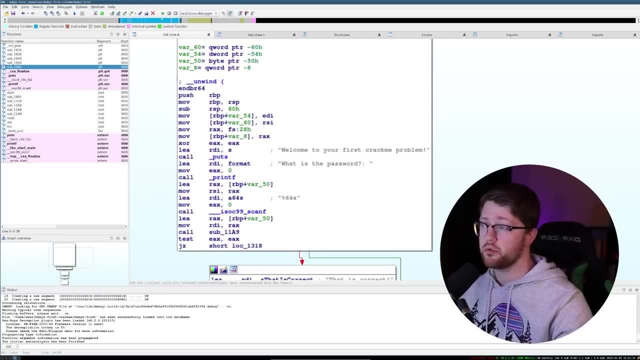 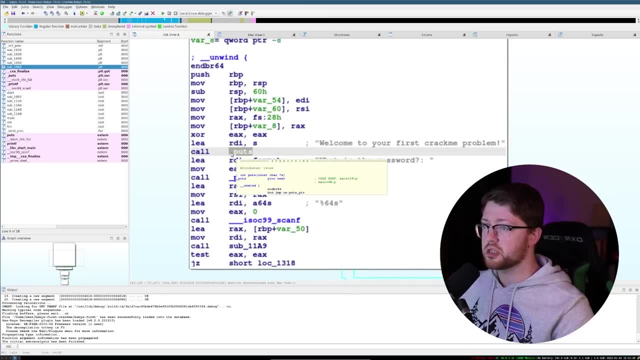 looking at the libc start, we didn't write any of that code. this is the code that we wrote, but the assembly for that code right, and we can kind of see that if we look at this we see we have the puts function get called and it gets called with this pointer to s in rdi, argument number one. 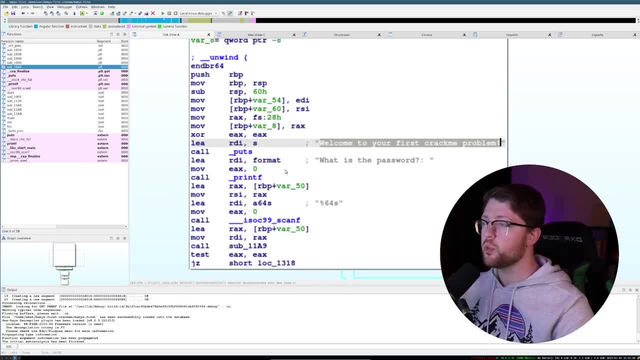 and that's where it says: welcome to your first crack me problem. we then have another one that says print f. print f is it gets called on the what is the password. so these are the two prints that get called to prep us to check our password, and then we have a. 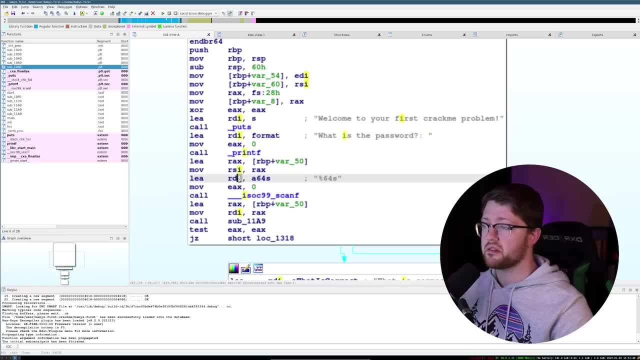 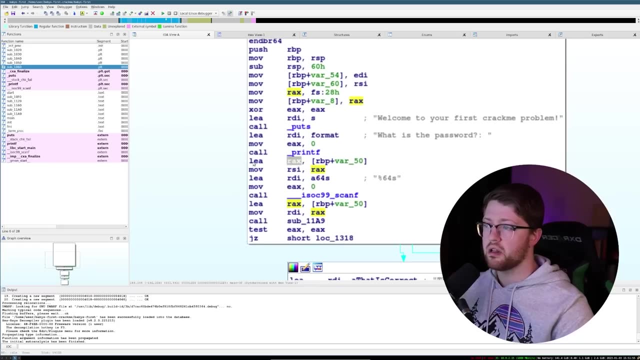 few things happen here. so remember how i said that the first argument is rdi and the next argument is rsi. well, we can look at this move instruction and see that rsi comes from rax. we're going to middle click on rax. these all get highlighted. rax becomes load, the effective address of this. 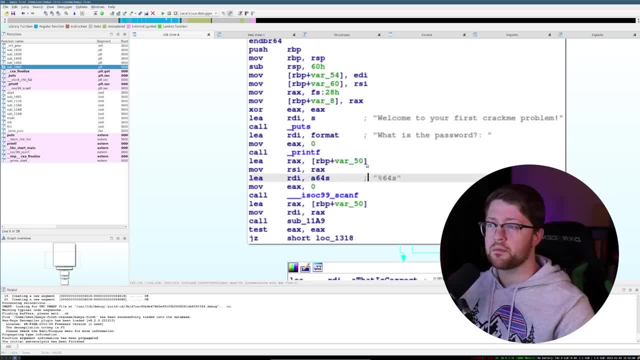 location here. interesting, what is that location? so, because it loads this location effectively, it actually puts a pointer to this location in rax before it puts it into rsi. so that means that this variable here, variable 50, is the buffer that we created for our buffer, remember we? 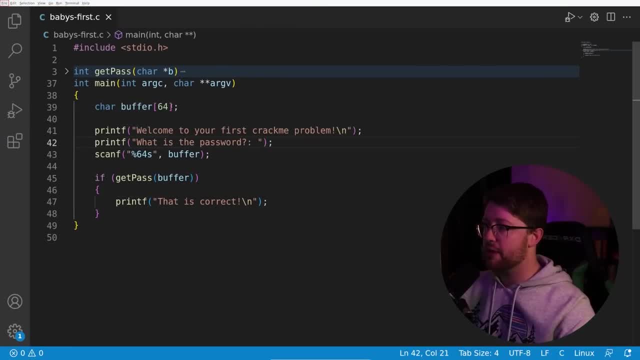 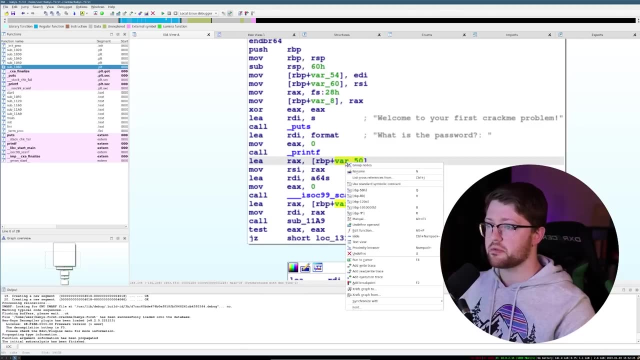 can go back and look at our code here. we created a 64 byte buffer, so that is the location of where our password is going to go into. okay, so let's go ahead, and we're going to label this. we're going to right click, hit name, we're going to type in buffer. by doing this, we are starting to infer more, and 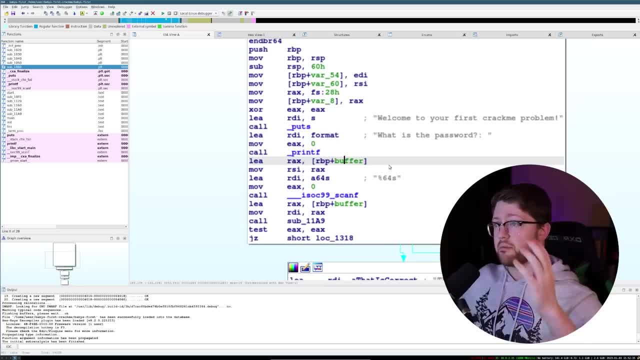 more of the information about the symbols that we wrote as programmers, that the malware wrote. the malware author wrote as a programmer of the malware, reverse engineering or whatever about what the program does. right, so we call the scanf function here, and then eventually we go down to this next. 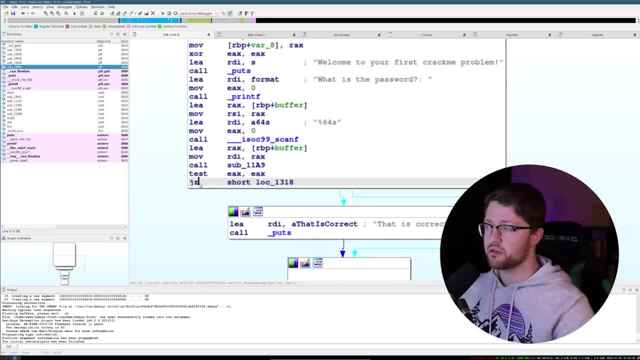 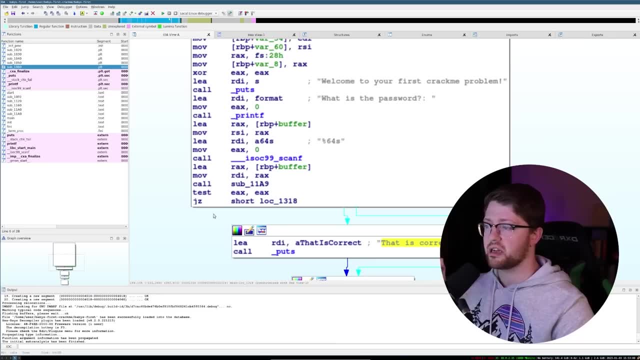 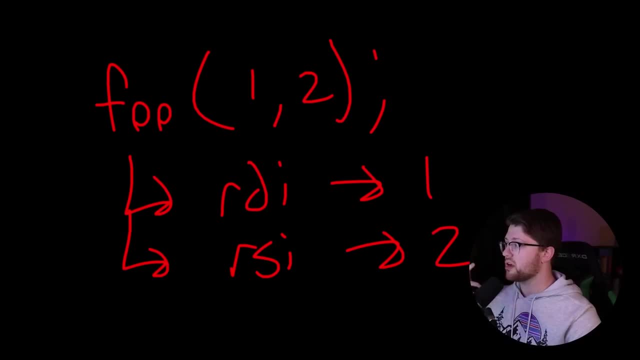 function here and then we have a conditional jump. we say jump z or jump zero to either this location. that is correct or something else. we're going to talk about how how that all works in a second. here we're going to take the current data that's going to be in this list and we're going to call it right. 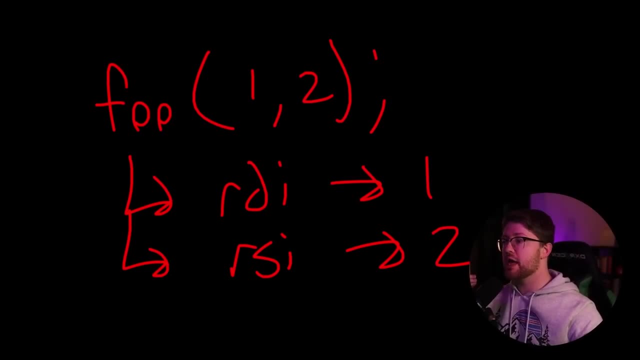 click, get into the to constant function and we'll call it rx and we're going to see that it's going to ask us that this is what we want. so what is it going to ask us like? what is this constant function called? it's going to ask us that it's going to ask us to insert a new variable into rsi. 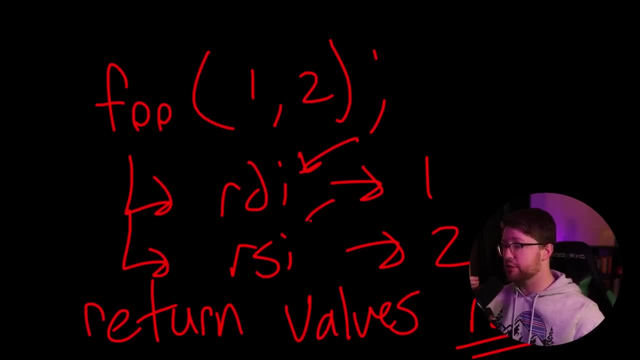 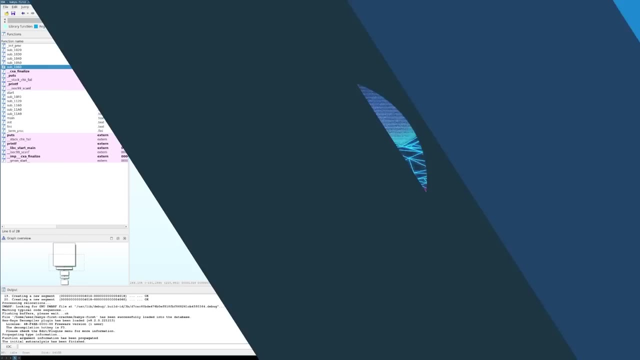 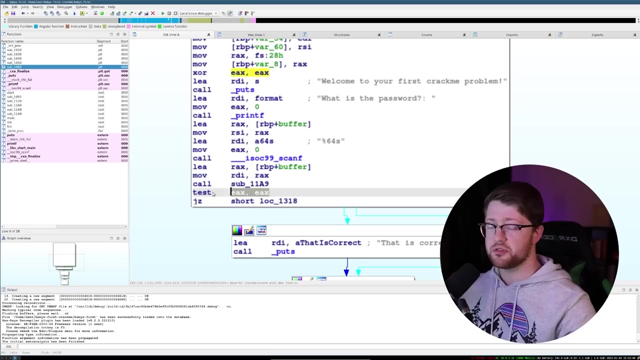 so we're going to press enter in the process. so we're going to use the data- you see that it's going to say else- and see if we can move this variable into an x or x and say, okay, I'm going to. We see that we call this function. the processor then tests EAX, which is the lower half of RIX. 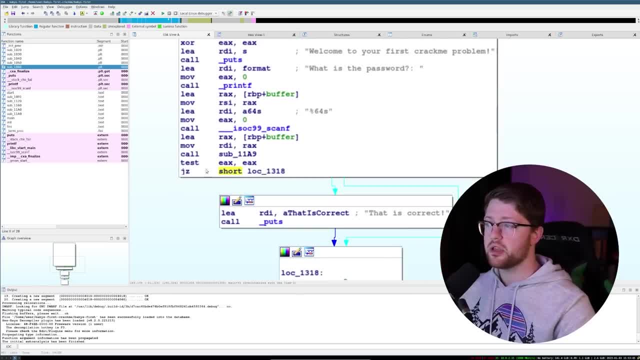 so it tests the return value, and if the return value is 0, we jump. the green line is where we jump on a positive test. so jump 0, we jump around this, and if it is not 0, jump 0, red right. 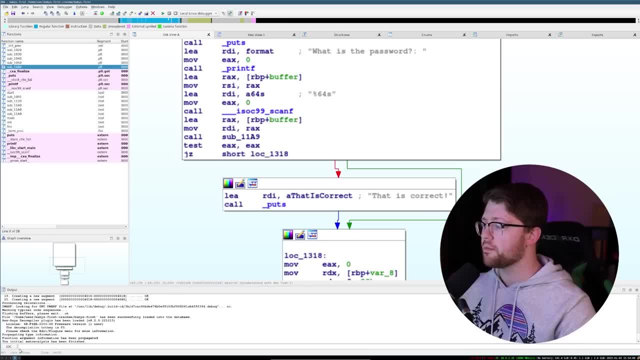 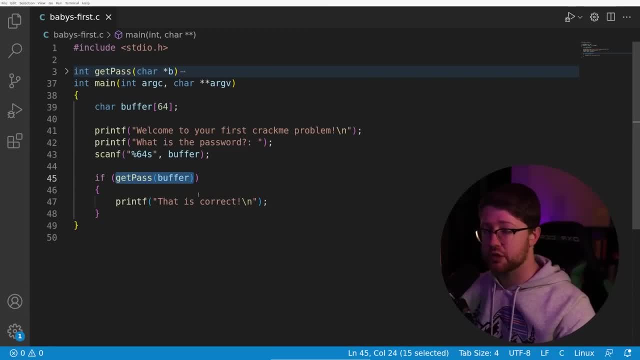 the red means we go here. it says that is correct. What is that coming from? If we go back to our code, we're testing the return of the get pass function. The get pass function will return 1 if our password is correct. and if it's correct we say that is correct. 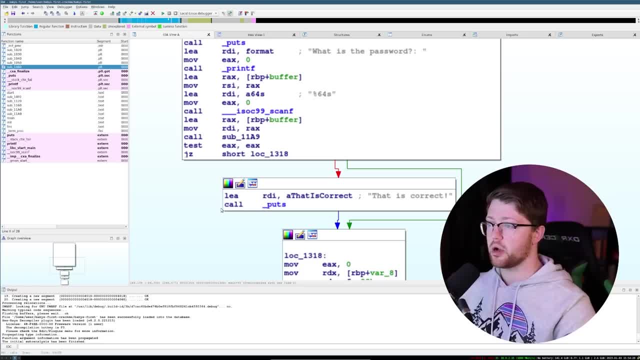 so that's how we got that out of the assembly. so now you're probably saying, okay, cool, let's get into that function, let's go figure out that password. okay, we'll get there. Step one: we want to rename this, the get password function. right, we can just kind of infer. 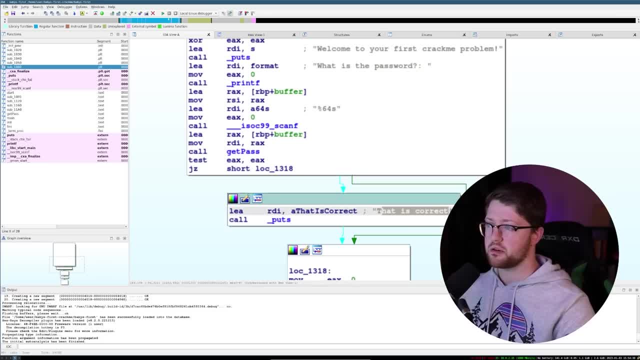 that you know. it says what is your password, if you get it right. it says that it's correct. we can just infer that that's correct. That is the get password function. so we're going to double click on that and here we have this. 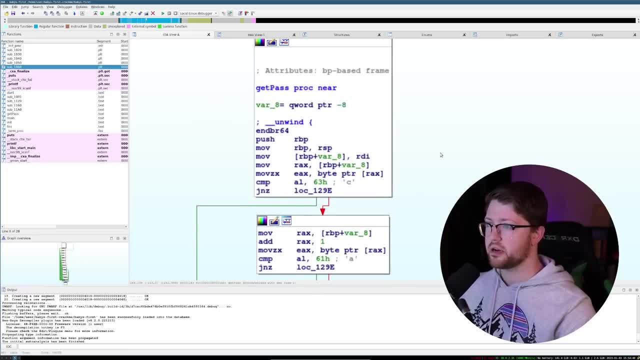 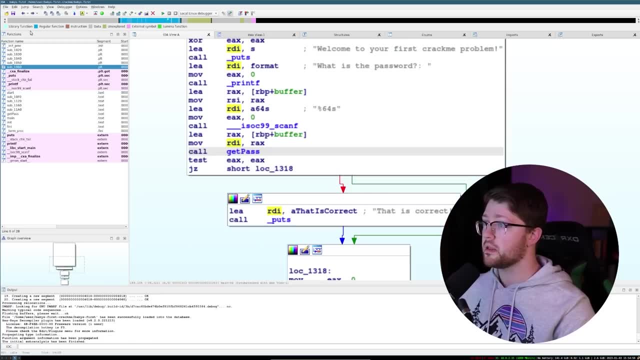 giant chart. You may already see the password starting to appear here. but remember what I said before: the RDI variable is the first argument that gets passed into a function. In this function here, we passed our buffer as the first argument, so we're going to go into there. 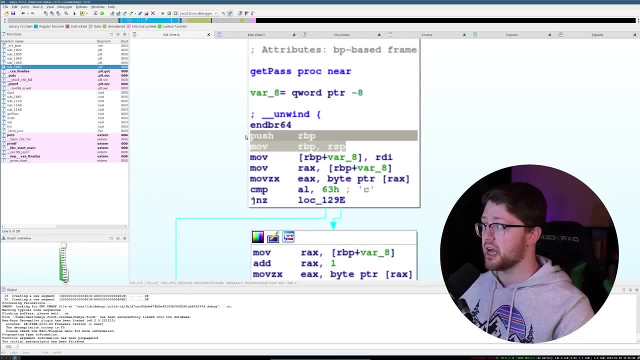 so if we look at this, it does a few things: it sets up our stack and then we move RDI- the pointer that we gave it as an argument- to another variable on the stack. The stack is preserving the argument, so we're going to call this buffer as well. 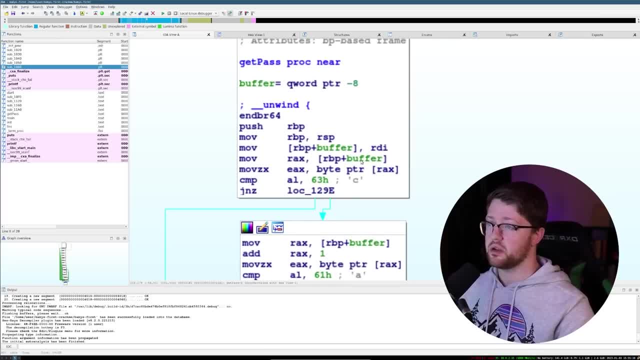 and this is a pointer- to the buffer. So now what it's doing is it's going to take that same buffer, it's going to put it into RIX and it's going to compare the first pointer or the first byte. so it's a treat RIX as a pointer. 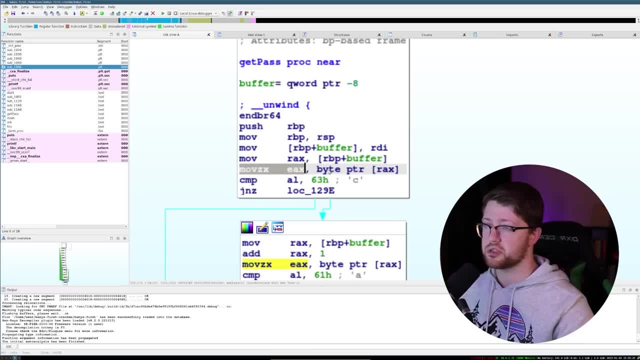 extract one byte and put it into EAX. that is what this instruction turns into, and we're going to compare that. AL is the lower eight bits of EAX and RIX. these are all the same registers, Just different parts of it, and we're going to compare that to 63H. well, as Ida is already showing you, 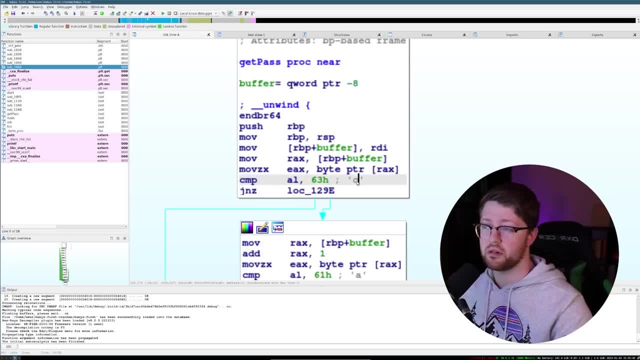 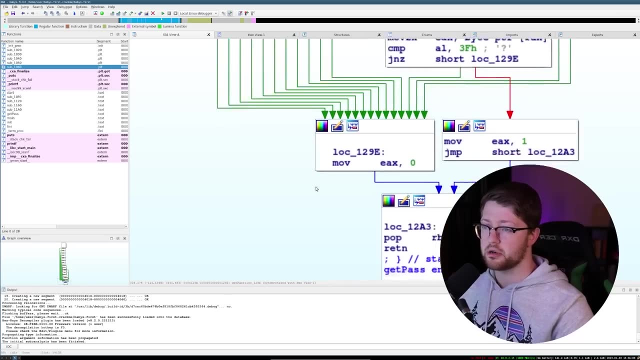 Ida is showing you. hey, by the way, 63H is the letter C. if that is not zero, right? If they're not the same, a zero comparison is also the same as the same comparison. so if they're not zero, meaning that they're not the same, jump away. and this is the return right. 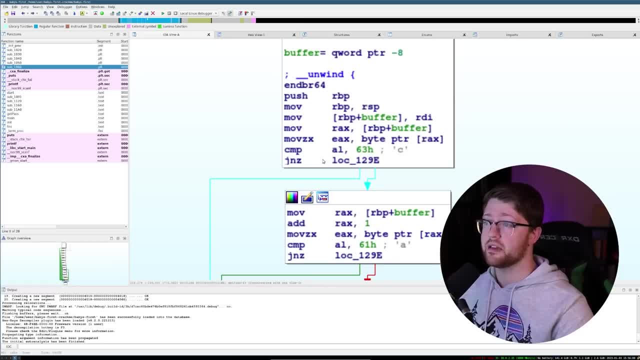 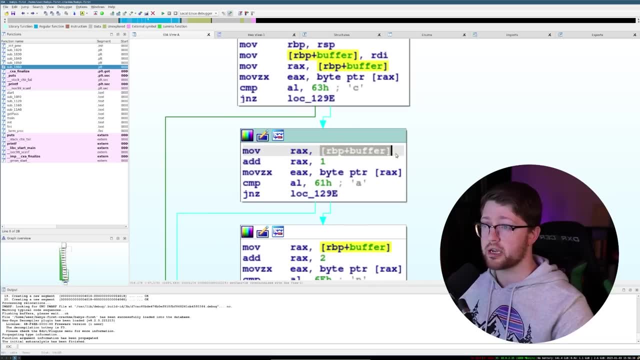 We are returning zero. so if we go back, if it is not zero, or if it is zero, meaning that they're the same. go to the next. add one to our pointer right. Extract the buffer, add one to it, which means increment, to the next character. 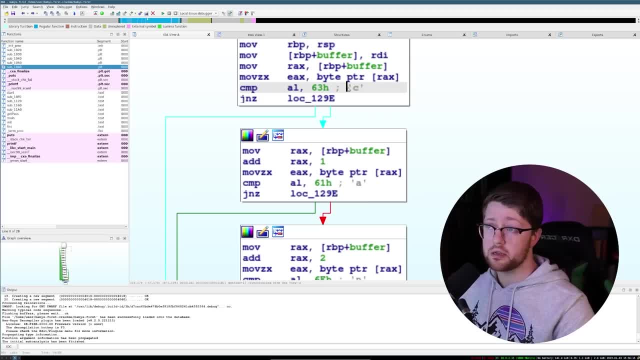 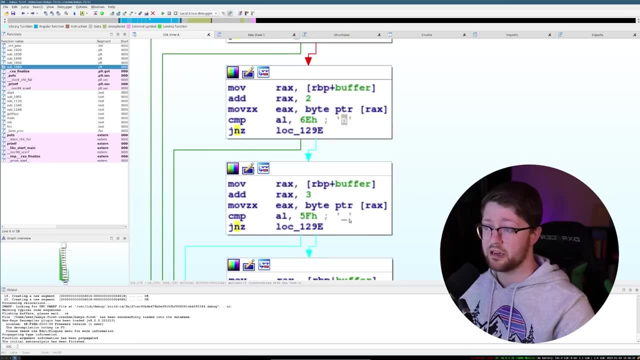 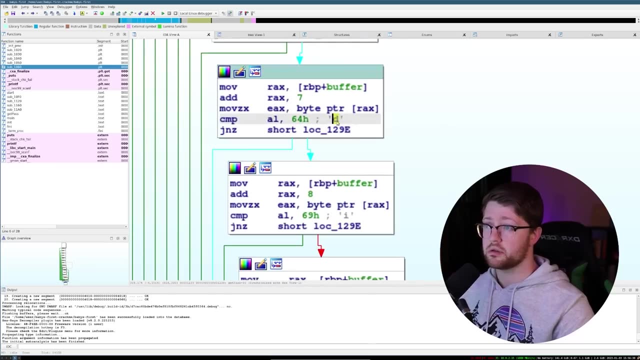 and compare that to the letter A, So we can actually just read the instructions here and figure out what our password is. so C-A-N- okay, that's a word- can underscore, ya, underscore, canya, underscore, dig, underscore. 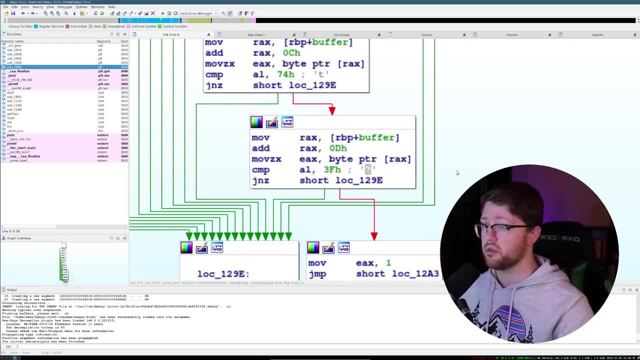 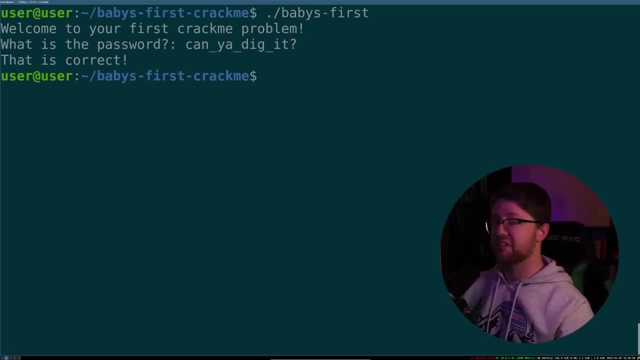 it question mark. okay, cool, so that seems easy enough. let's try it out. Can ya dig it? That is correct. What did we just do? We took a binary that we didn't have the source code for, and again we did. 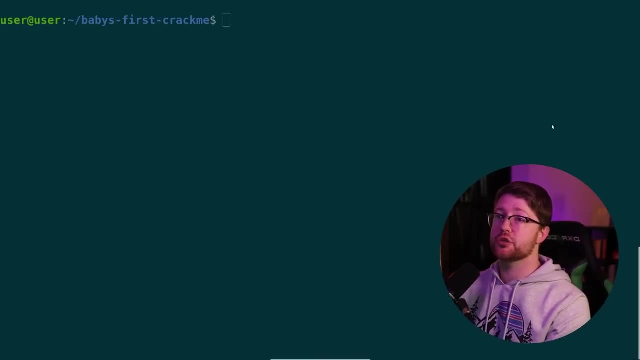 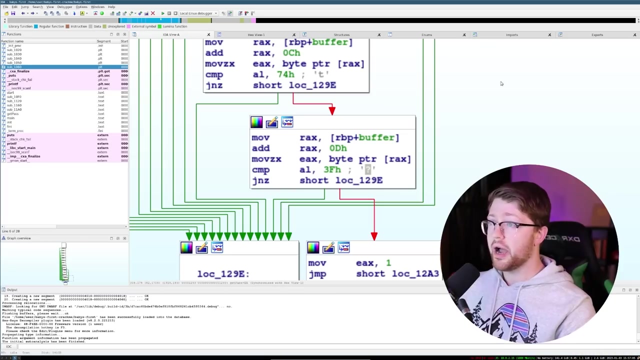 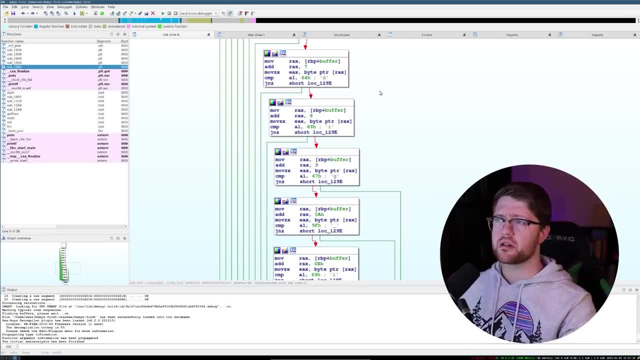 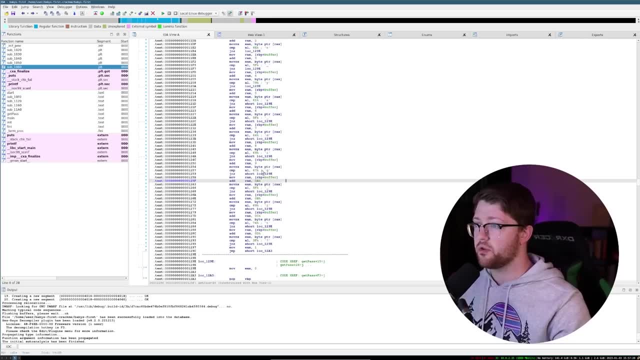 and eventually the password. You may be asking why did strings not reveal the password in that binary? The reason was, when you look at this, the actual hex code for the binary is the instructions. at that location, The comparison to the letter G actually gets packed into the instructions. 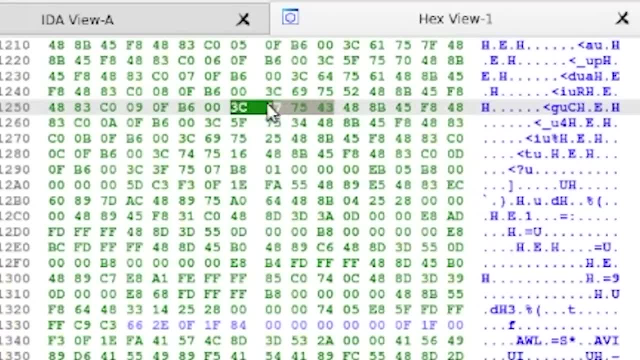 If you look at the instruction here you don't get to see the letter G packed into the binary. Actually you kind of do. You can see the letter G here gets packed into the instruction because we're comparing that byte to the letter G.